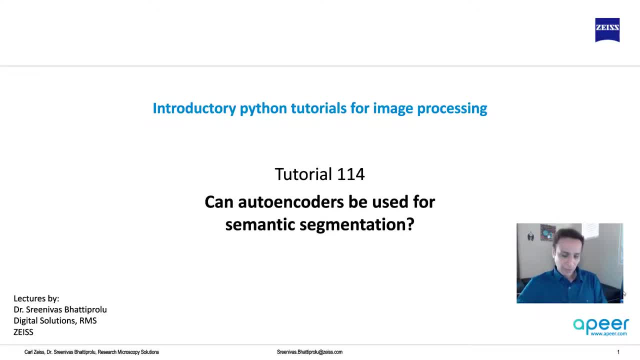 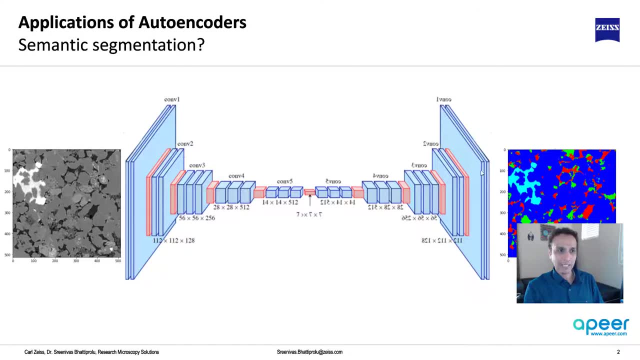 smaller vector into your original image. So in fact, let's go ahead and have a quick look at it. So you have an encoder path on the left hand side and a decoder path on the right hand side. That's kind of symmetric to your encoder path, right. I mean, in this graphic I literally flipped this. 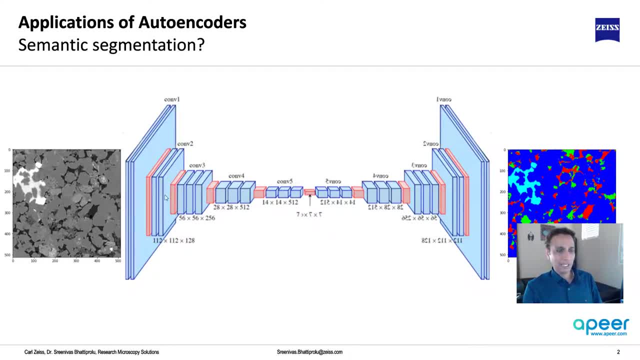 image and then concatenated or added, I should say, to this left hand side. So my image on the left hand side is reconstructed as image on the right hand side, And in the last video we left off by asking a question: can we trick this? Can we use the auto encoders for semantic segmentation? I 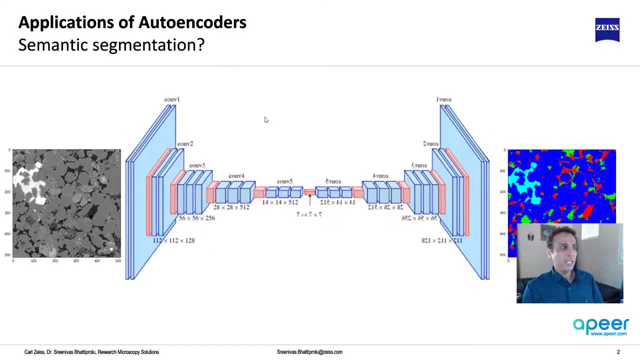 use the term trick, Because auto encoders typically mean you have an input image and you're reconstructing the same input image by going through this architecture. Now, instead of using the same input as your expected output, what if we provide a segmentation mask as the expected output? Can we teach an auto? 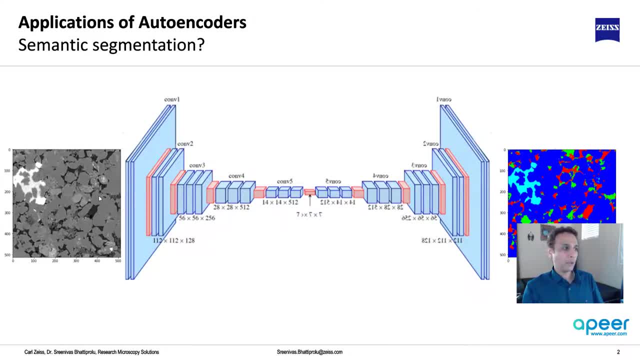 encoder to learn this mapping from your original input to a segmented output. If that's the case, then we can do our semantic segmentation using our nice architecture that we are displaying here. okay, So let's jump to some code to literally do this experiment by providing: 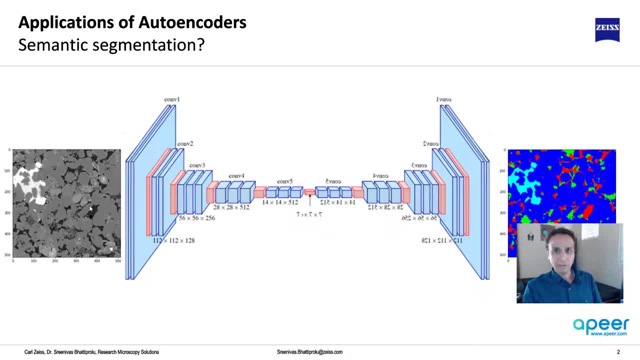 our model, our auto encoder that we have used already in the last video- the same one. Instead of providing our x and y to be the same, let's provide our x and y to be different: X as our input image and y as the segmented mask. 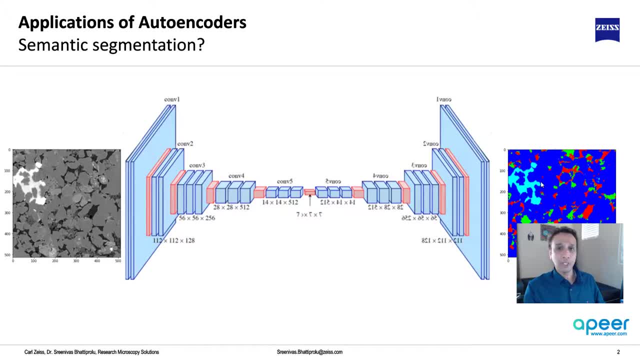 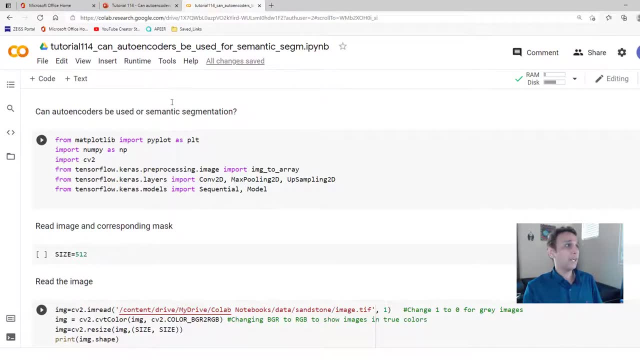 And let's see if that is acceptable. So let's jump into the code. Okay, as usual, I'm going to share the code with you, So don't worry too much about writing it down right now. One quick note: I am. 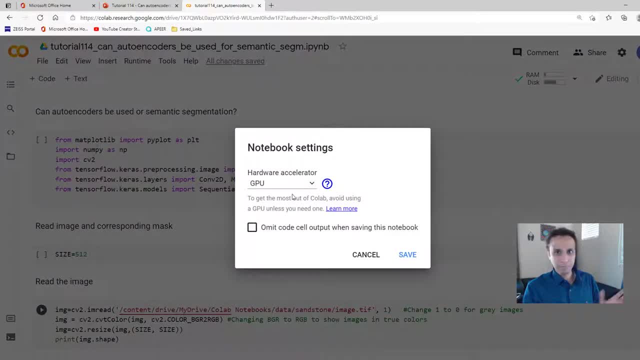 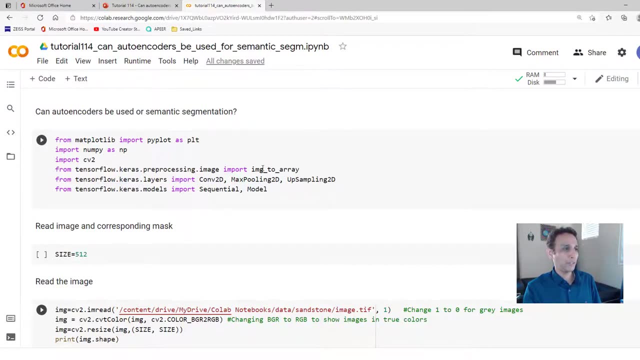 using GPU on colab. thanks to Google, we get this for free, So please go ahead and use it responsibly. Do not just do a bunch of, do not hog the GPU resources, because everyone needs it. Okay, now few lines. i explained it again in the last video. we are just importing the libraries required. 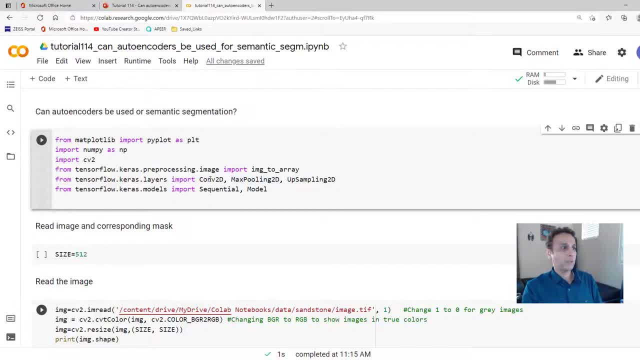 libraries and going down the encoder path. we are going to use convolutional layers and, more importantly, max pooling. so we are going from a larger size slowly down and to reconstruct it back. in this example we are going to use upsampling 2d, although you can use convolutional 2d transpose. 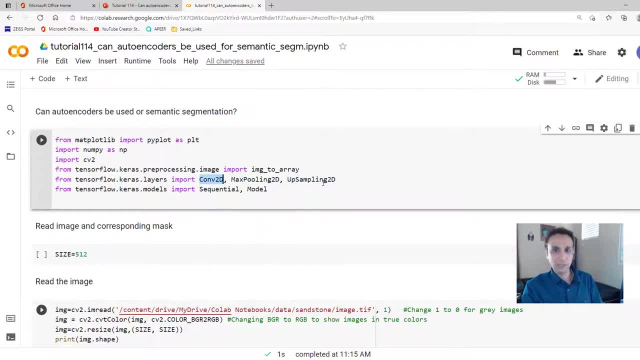 which is exact opposite of con 2d, like the name suggests. okay, i'll talk about that in the next video, just to give you some clarity on what the difference is between these two. and we are going to use sequential uh method to create our model. we have been using that. 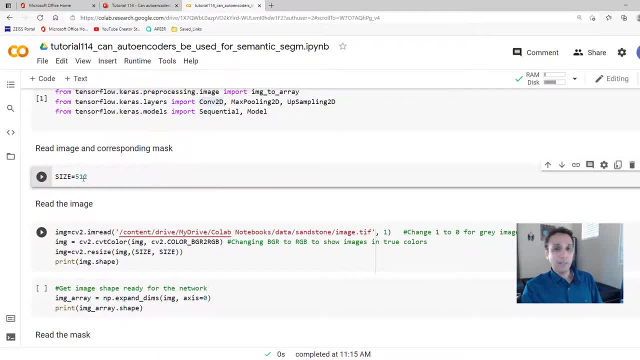 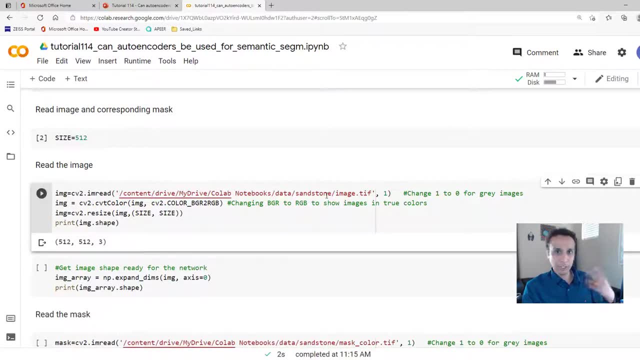 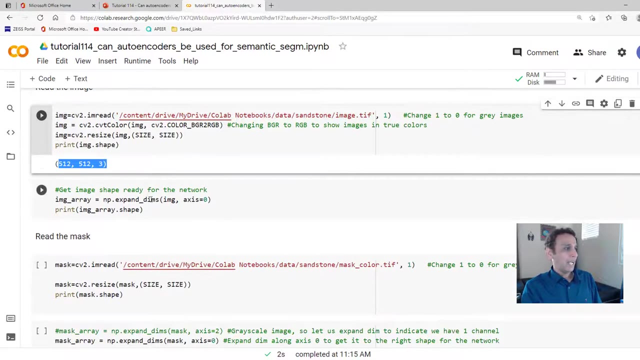 anyhow in keras. okay, so let's define our size to be 512, let's define a larger image and let's go ahead and import. i'm going to load a sandstone image that i showed you earlier as part of the presentation, and the size of that image is 512 by 512 by 3.. and let me 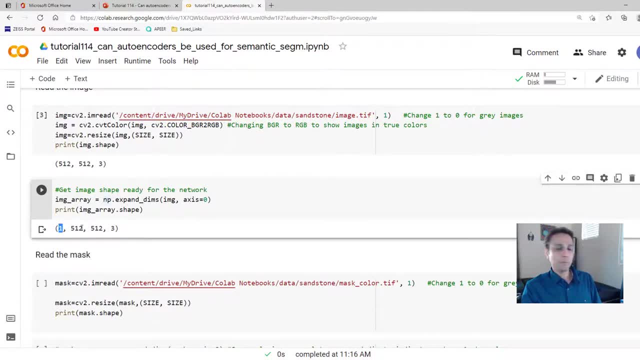 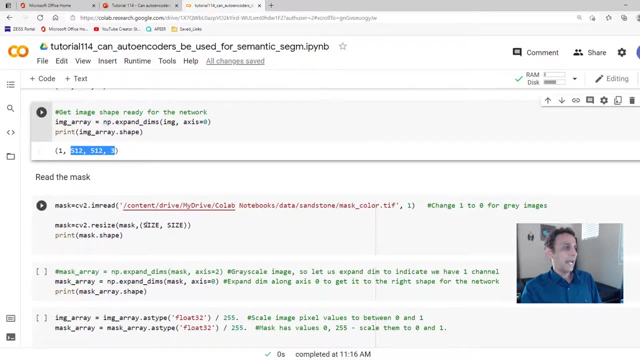 expand, expand the dimensions by one just to make it ready to go into our neural network. so one image of size 512 by 512 by 3.. and now comes, uh, the mask part right. so we are tricking our auto encoder. last, in the last video, we just said, okay, that's my image and my x is image area, my y is: 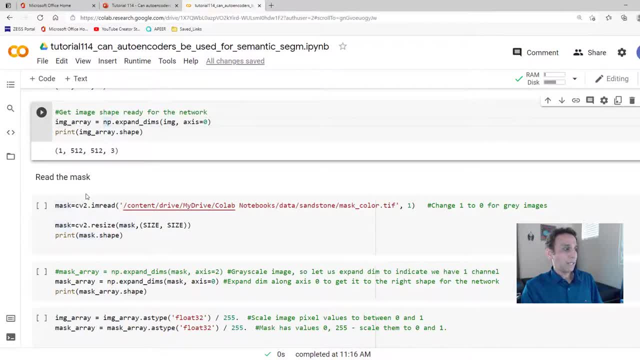 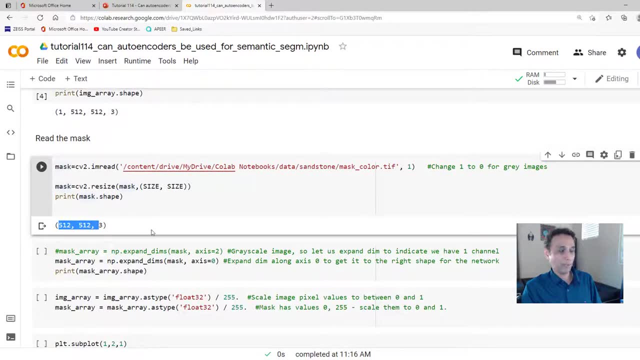 imagery. okay, so do the mapping one on one. but right now we are going to load our mask and then get to the same shape. right now we have 512 by 512 by 3, right, and that's pretty much the same size, right, 512 by 512. 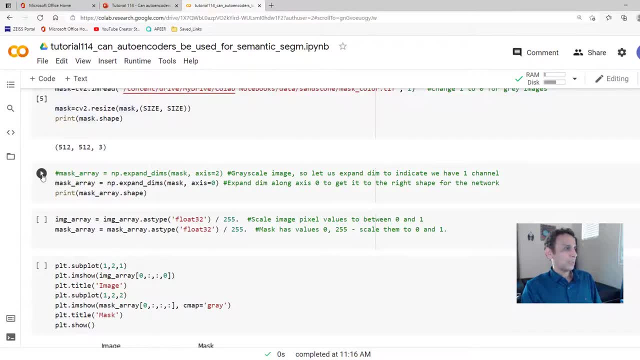 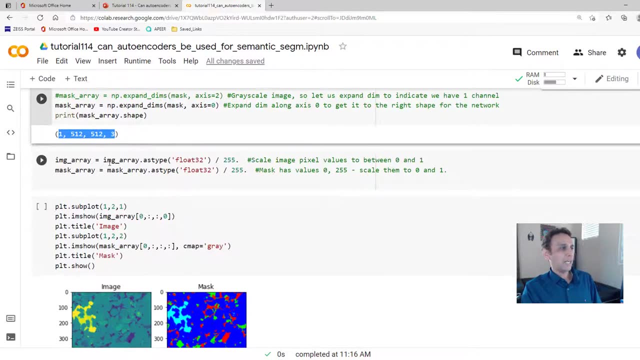 by 3. they need to match up, okay. so now we are going to expand the dimensions of our masquerade again to get it to 1, 512 by 512 by 3, and finally i am dividing both my image and mask by 255.. why? 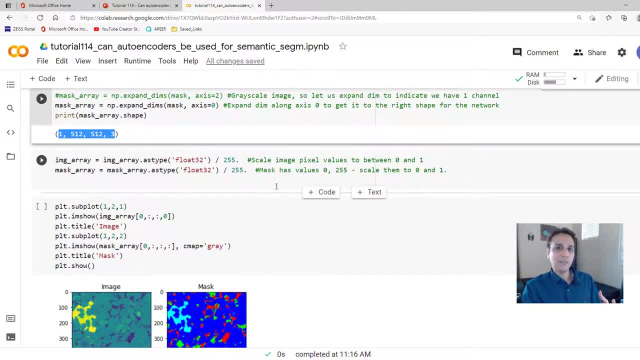 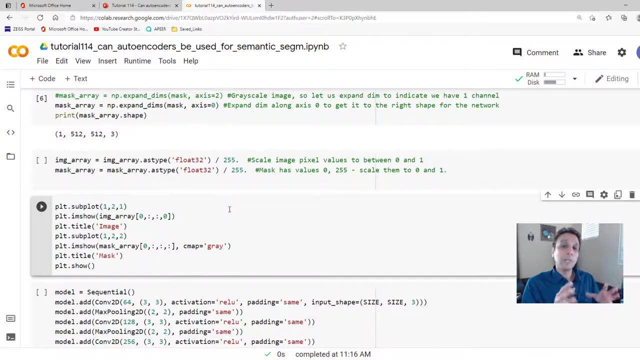 am i dividing my mask by 255? because my mask has values ranging from 0 to 255 and by doing this, well, my mask has different regions. let's close this. my mask has different regions of values that come fall between 0 to 255. by dividing those by 255, i'm just bringing 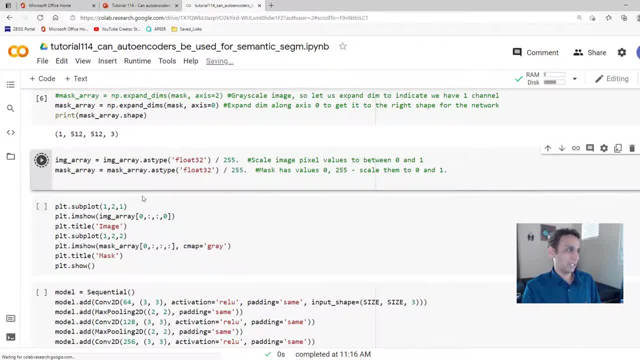 everything to values below 0 to 1.. that's pretty much it same for images. if your masks are already like 0, 1, 2, 3, then you don't have to do anything. even in this case, if i don't divide by 255. 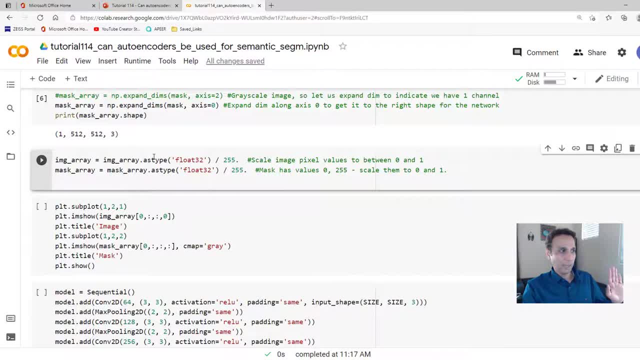 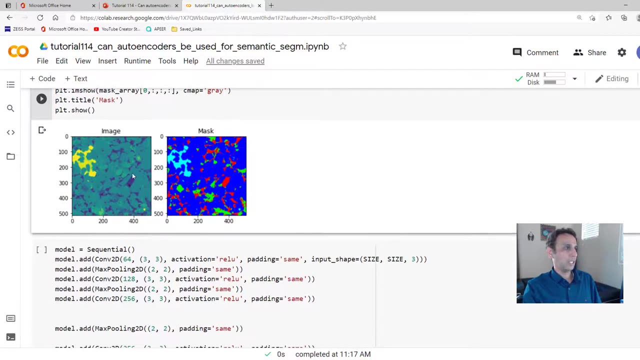 nothing wrong. you need to divide your image area because that's what you're training on and the masquerade is just what we are trying to predict. okay, so, but i'm doing this just for the fun of it. okay, let's go ahead and plot our image and corresponding mask. there you go. so that's my 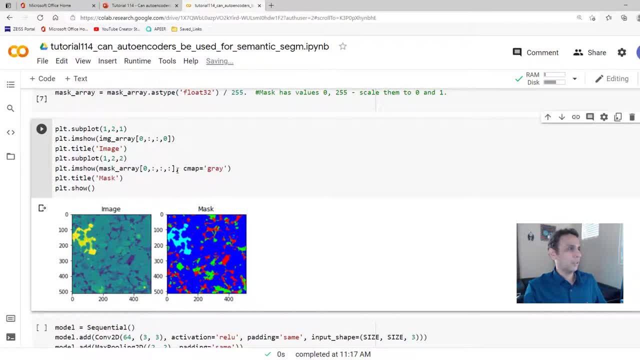 input image i thought i put. cmask is equal to oh wrong one. sorry about that. i had to do that right there. i don't like my image to be in pseudo colors. there you go. that looks realistic now, right, so this is my image. this can be think of this as a xrm image. x-ray micro. 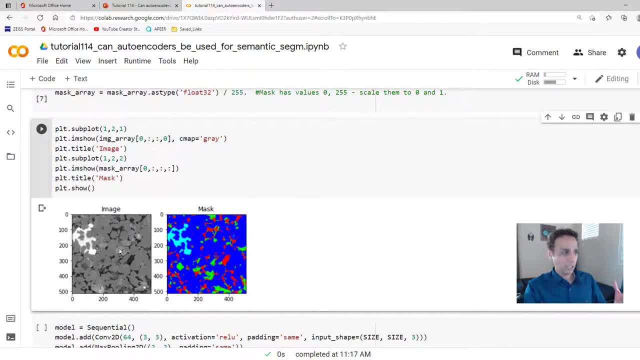 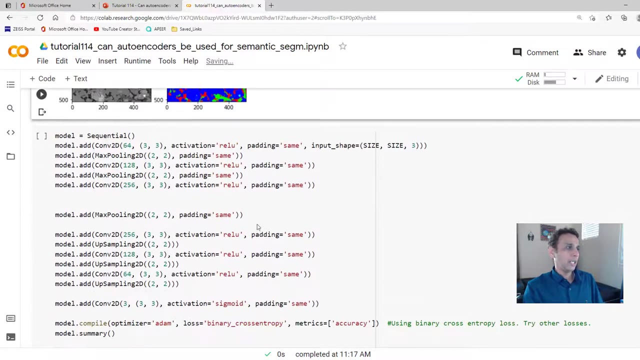 scope or a ct computer tomography, one slice out of this tomography data set. or this can be an electron microscope image, but it doesn't matter, it can be even light microscope image. it's just an image, and or even a satellite image. right, an image and corresponding mask. okay, so far, so good. 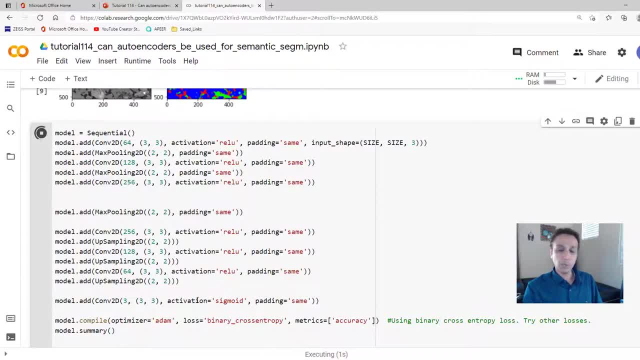 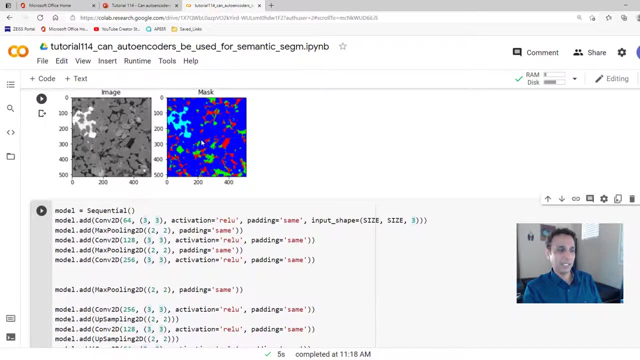 now let's define our auto encoder. this is exactly the same what we have done in the last video, right? so 64 uh filters, 128, 256 and progressively, symmetrically, going back down with an output of three channels. why three channels? because my label in this case is a rgb image with three. 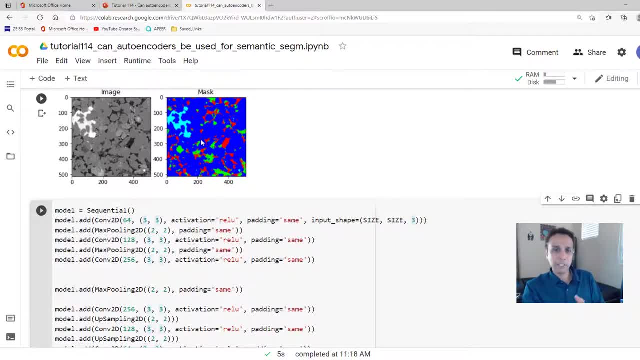 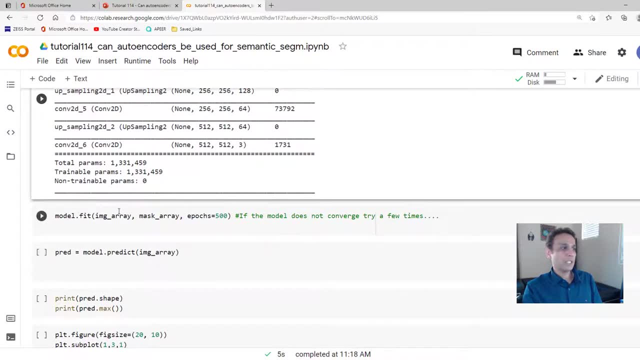 channels. if it is just a grayscale image- 0, 1 to 3 pixels- then that output would be one right there, okay now? uh, yeah, so we have that, and next we just need to fit the model. remember, in our last video we did image array and image array. now let's go ahead and do image array and mask array, okay, and 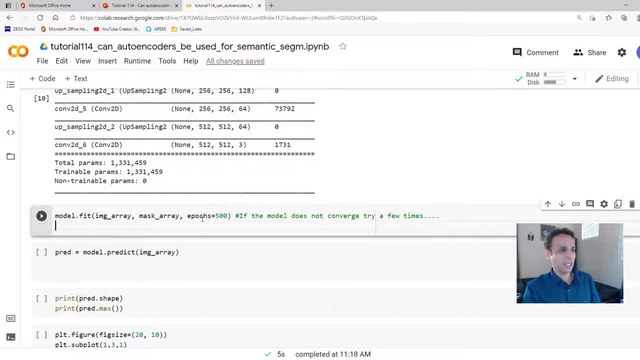 let's train it for 500 epochs. if the model is the same as the image array, let's go ahead and do image array and mask array okay, and let's train it for 500 epochs. if the model is the same as the image array, model doesn't converge, let's try a few more. but let's go ahead and train this for 500. 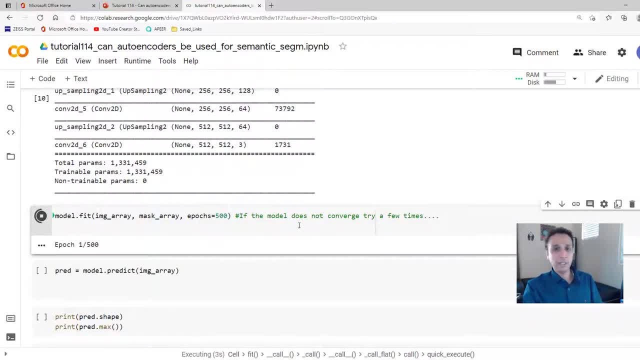 epochs and see what we get again. as usual, i'll pause the video until this is done so we can see if we need more training. if so, i'll pause again. but let's give this a chance. in the last video we did 1000 epochs. right now we're doing 500. so once it starts it should be relatively quick, but but. 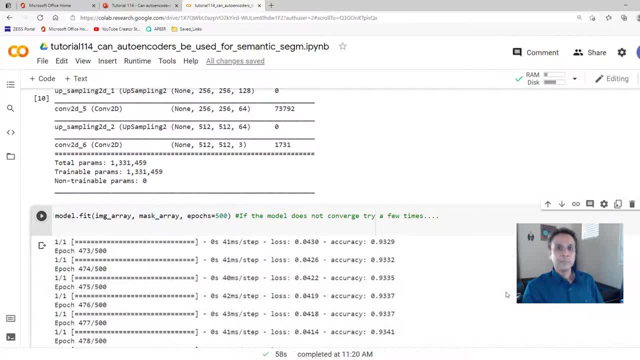 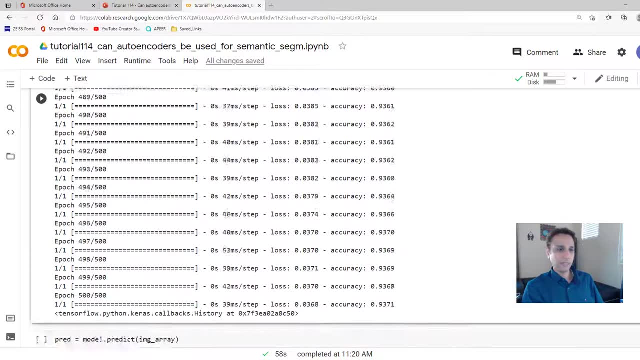 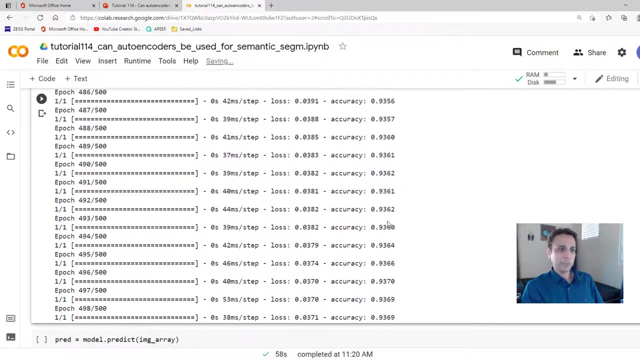 let me pause the video and then continue. okay, so this is done and giving us pretty decent accuracy. actually looks like it's saturated about 93 right there. so even if i continue, i'm not sure if i'll get any better than this. you see, the last few of these epochs i should have plotted, but that seems to be. 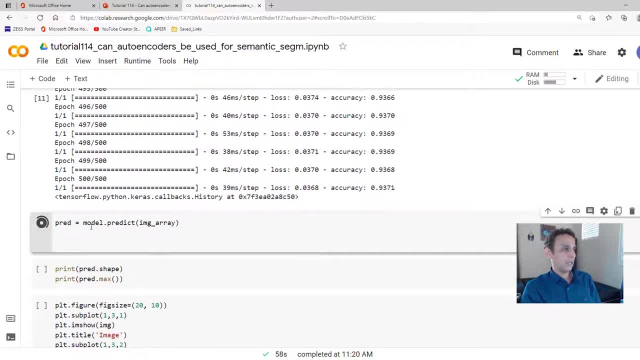 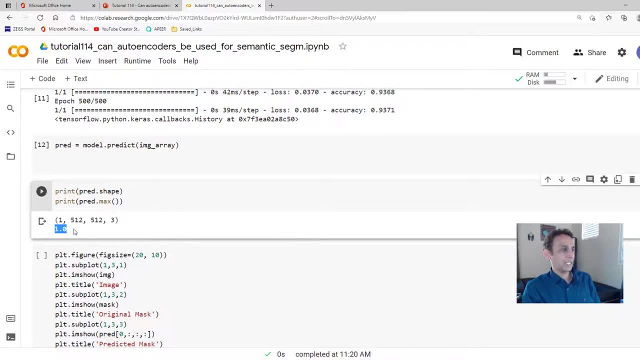 uh, saturated right there. so let's go ahead and predict on our model and first of all, let's go ahead and see the maximum value right there: one, yeah, that makes sense. uh, my prediction, because again we normalized everything to value 0 and 1.. that's just a quick check, a sanity check that i 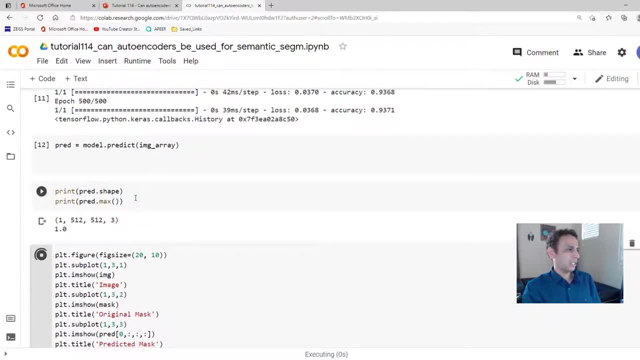 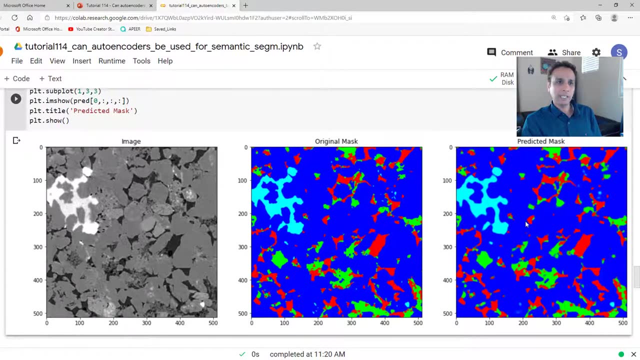 added over there. so let's go ahead and plot it. so let's plot our input. there you go. so this is my input image and this is the original mask and this is my predicted mask. that's not bad at all. right, that looks very good. so the answer to our question- can we use auto encoders for semantic segmentation? is maybe. 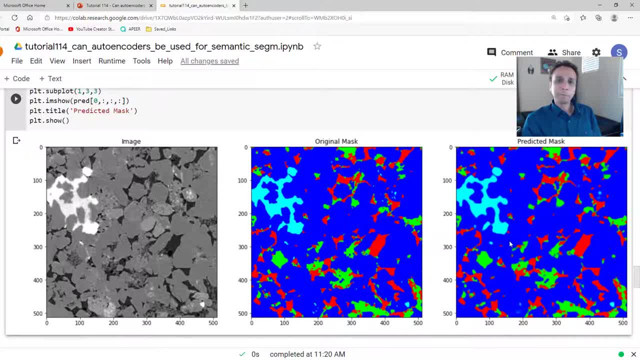 why do i say maybe if this looks so great? well, even when we reconstructed our image in the last time we did auto encoders- when we view the input as using auto encoders, we had an extra input in one video- we saw that we lost some resolution and you can see that here. you see very nice sharp edges. 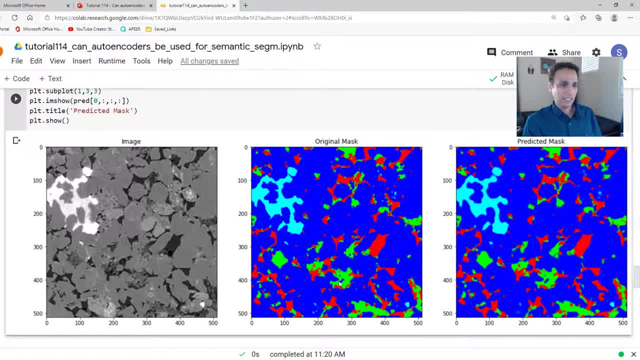 a lot of like if you look at the details in this region. yeah, you see, look at that small void right there that shows up as like some blurred region. look at this void right here. look at the same thing over here. i mean on first look, it looks like we are getting. 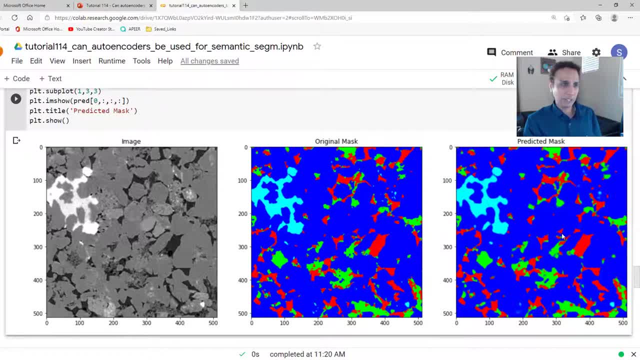 very good segmentation. yeah, of course i agree with you, this is not an easy sample. uh, to segment this is great, but look at all the rounded edges and this is: we are using the same image and same mask and we are predicting on the same image. so we should get the same mask. but if 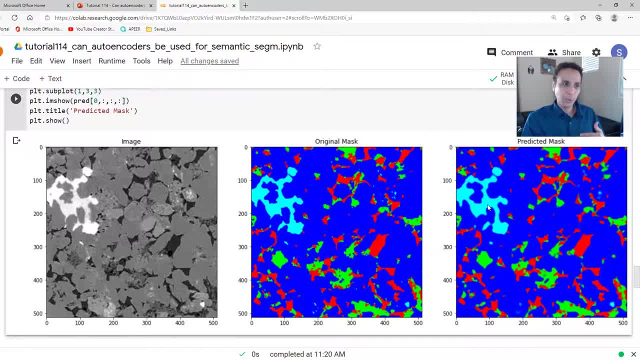 you expand this, uh sorry, if you extend this to a whole bunch of images and you're training it and you give it an unknown image, how does the segmentation perform? well, it actually performs in a decent way, except it's limited by the resolution. why? because we are going again from a